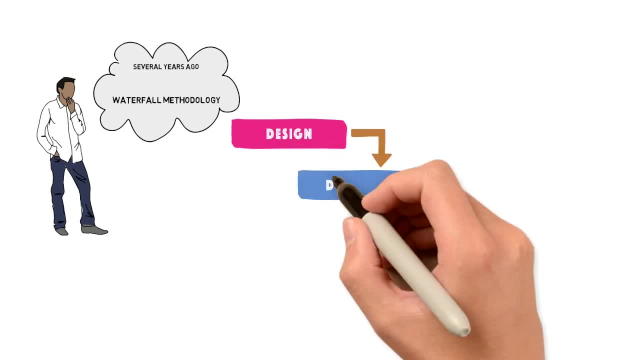 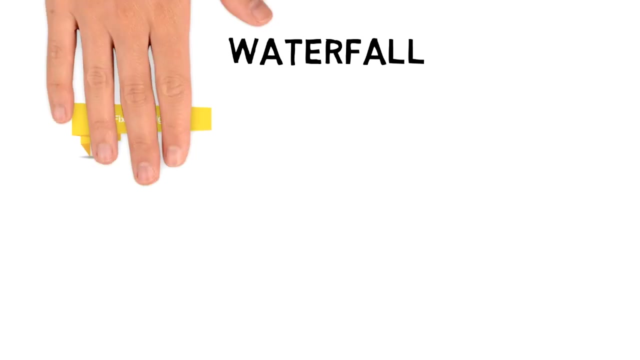 way Progress flows downwards in one direction, like a waterfall. Each of these phases represents a distinct stage, and each stage generally finishes before the next one can begin. Waterfall was organized in such a way that projects had to be finished within a certain budget fixed scope. 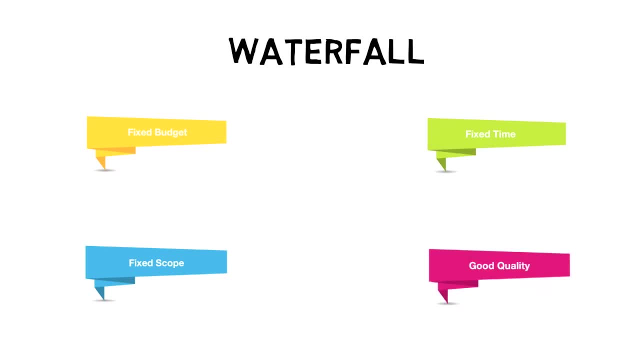 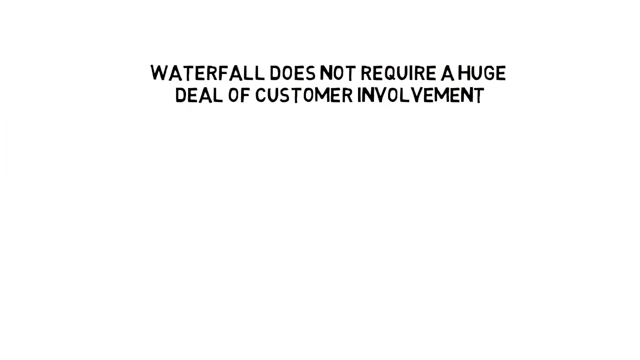 fixed time and good quality, which was almost never the case, and the customer was always unhappy. In fact, even when the project respected the budget, scope, time and quality, the customer was still unhappy. But why? As waterfall does not require a huge deal of customer involvement, so by the time, 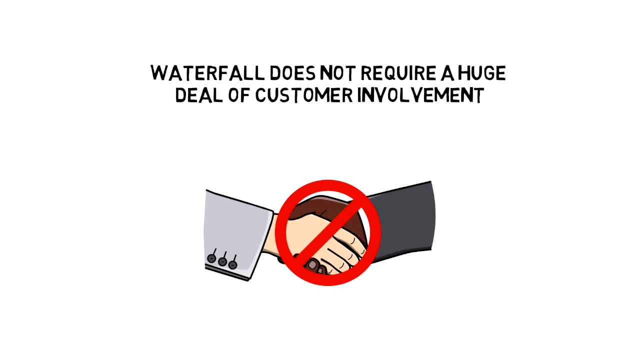 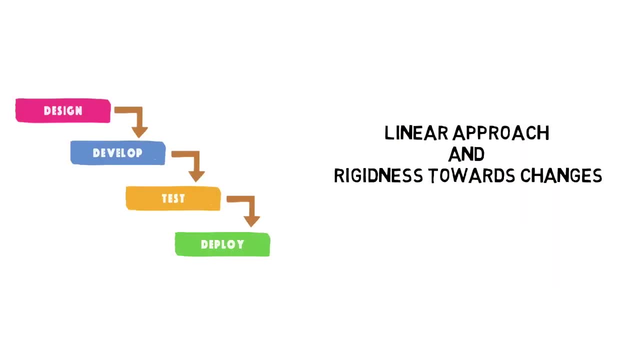 we deliver what we thought the customer needed. it's not necessarily what he needs anymore And because of its linear approach and its rigidness towards changes in the development of the product and the process, the project was able to continue. The customer was happy with the results of the. 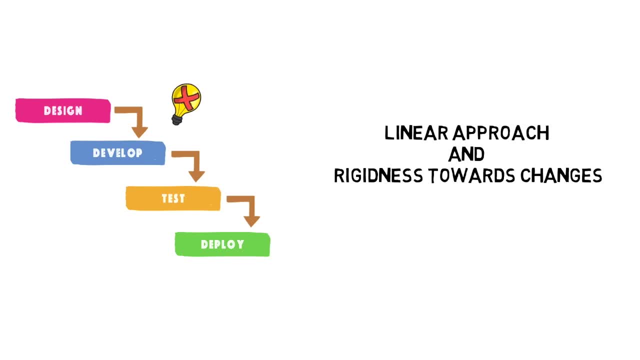 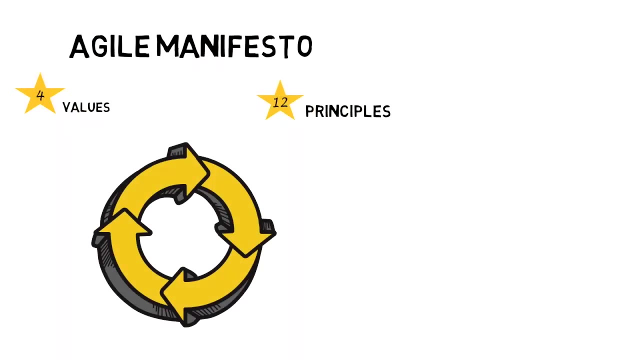 itself, it makes it almost impossible for new ideas to be included, which clearly impacts the customer satisfaction as well as the quality of the final products. agile came to solve these issues with the four values and the 12 principles. we create things differently in agile. we build products. 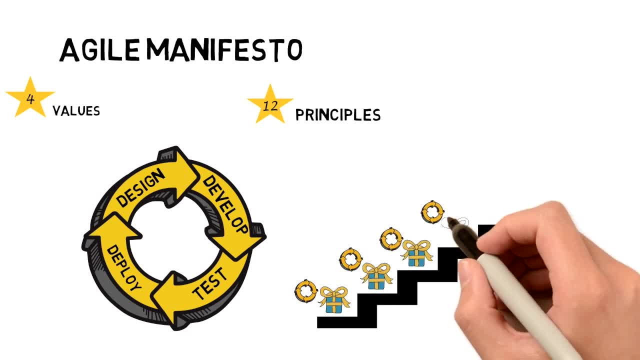 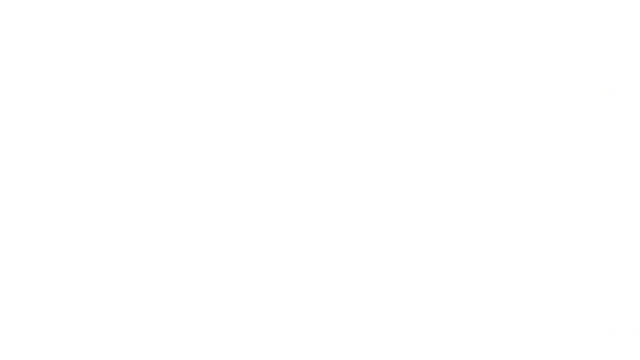 incrementally and iteratively, which helps teams deliver value to their customers faster and with fewer heads. instead of betting everything on a Big Bang launch, an agile team delivers work in small but consumable increments. we start with a small piece of work and we go through the design development. 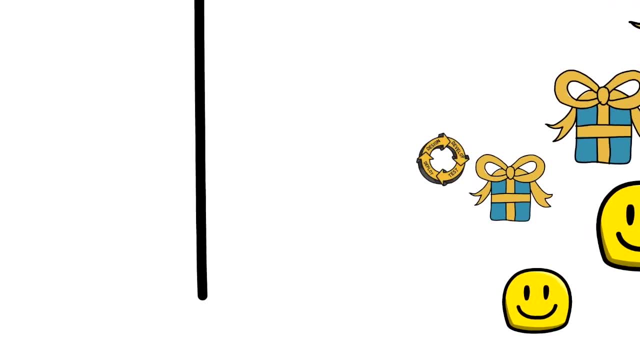 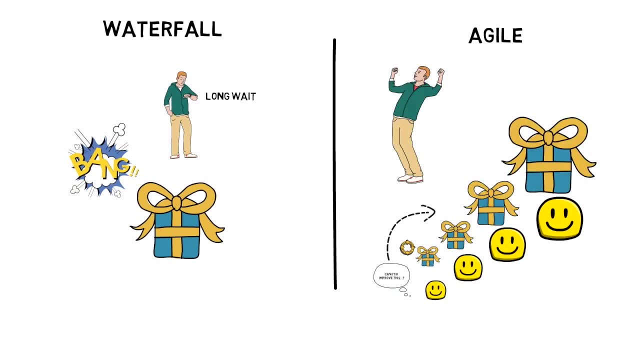 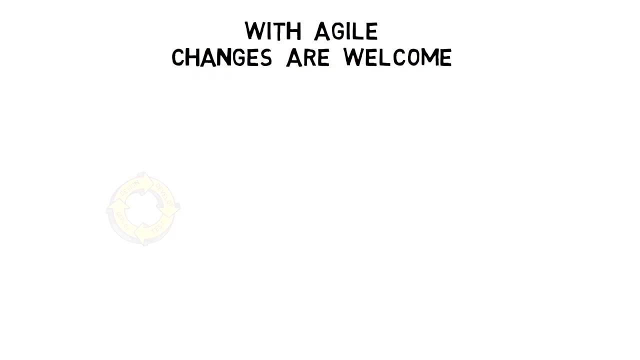 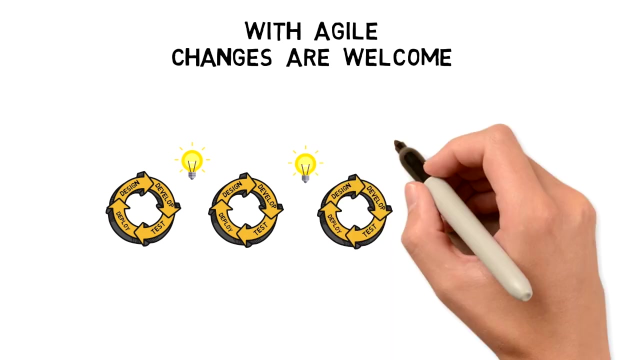 testing and deployment. the feedback from the customer and stakeholders is then collected and fed back into the cycle. with agile, changes are welcome. the rapid delivery of the value in small increments allow teams to change their products based on customer feedback, frequently and with lower costs. this helped them to keep up to date with the 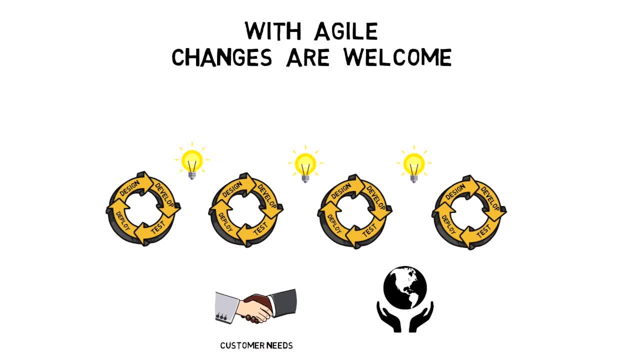 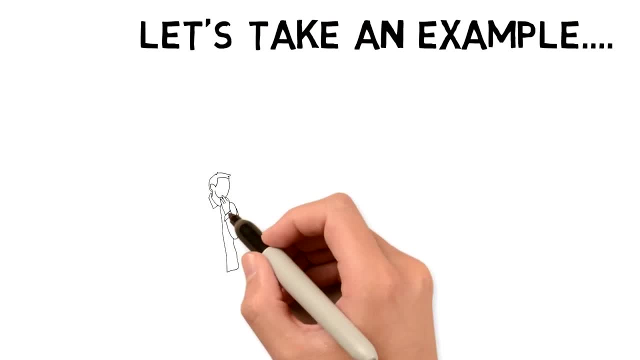 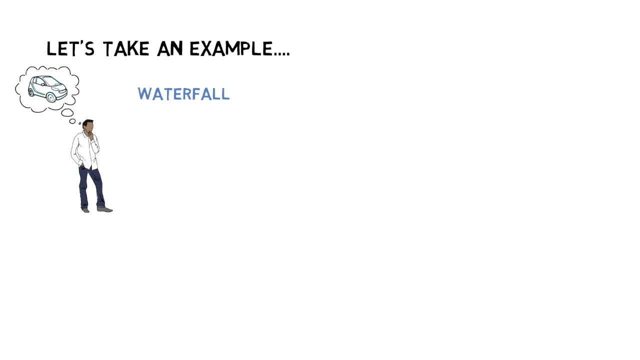 users needs and the constantly evolving world. let's take an example. our customer needs a car to be able to go to work. if we decide to build this product in a waterfall way, we will start by defining what the ideal car should look like after several weeks or month of thinking. 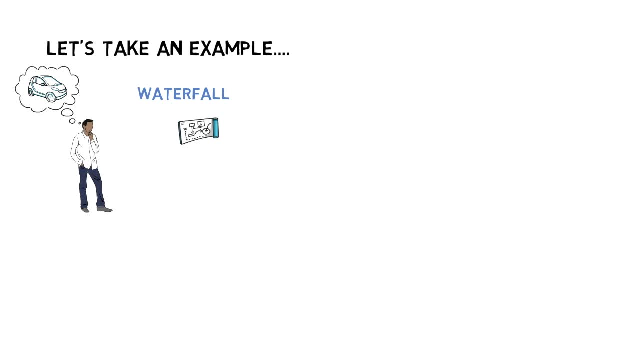 and once this phase is done we start building the car, first the wheels, then the engine, the frame. then we assemble everything and deliver it to the customer. what happens here is that during the first phases the customer is not receiving anything for a long period of time. If we are optimistic, he is happy with the car you gave him. but the customer might say: 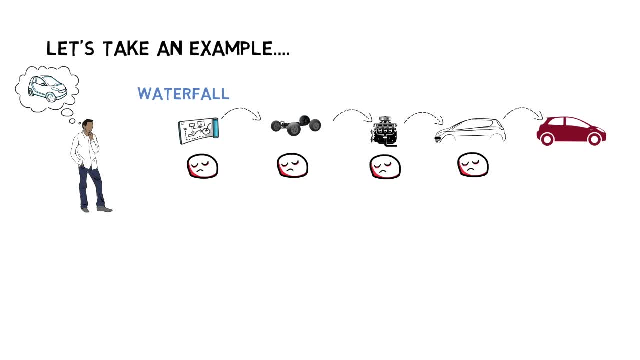 that this is not the car he was expecting and he doesn't like this design. In this case, changing the design will be very expensive. If we decide to build this car in an agile way, we will involve the customer on a regular basis and we will ask him for input and feedback while building his car. 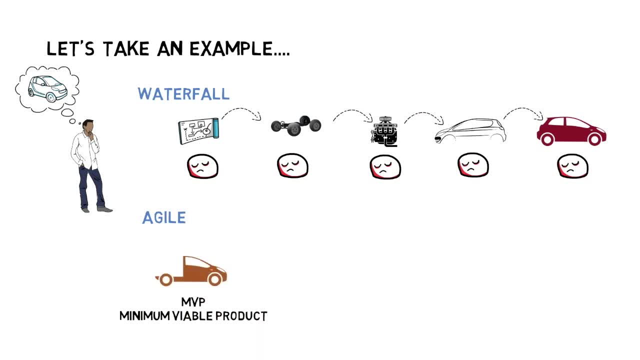 We can start with the minimum viable product, the least expensive product that can allow us to test our idea and for him to try it. Based on his feedback, we can improve it and add new functionalities. At the end, and as the customer was involved all the time and his feedback was act on, 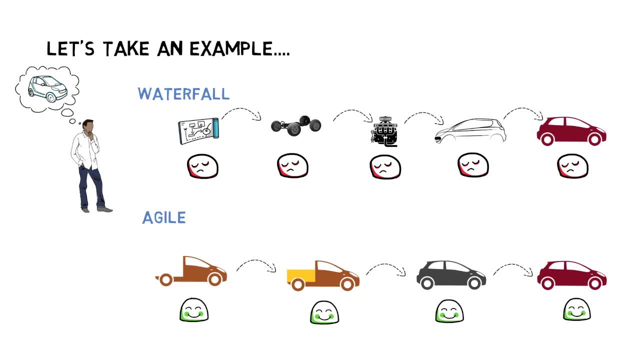 we know we are delivering exactly what he expects. There is one important thing between these two ways: In waterfall, we cannot stop before we deliver the full product defined at the beginning. In agile, as we are delivering each iteration a functioning product, the customer might 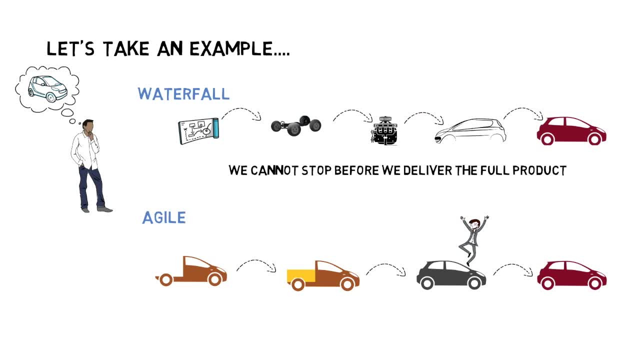 say that he is happy with what you just presented and he doesn't need more, so we don't have to spend more money to add additional features that the customer doesn't need. As a summary, One of the most notable differences between agile and agile is the fact that the customer 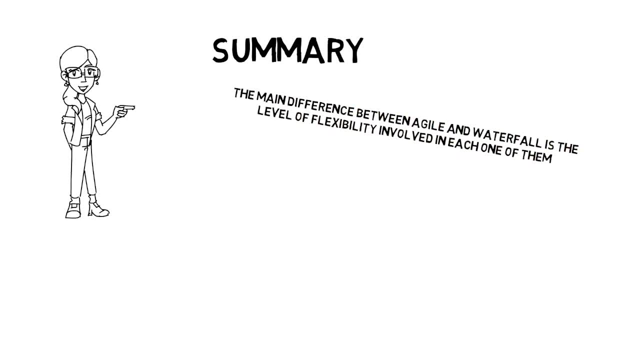 is happy with what you just presented and he doesn't need more, so we don't have to spend more money to add additional features that the customer doesn't need. Another important difference between agile and waterfall is the level of flexibility involved in each one of them. 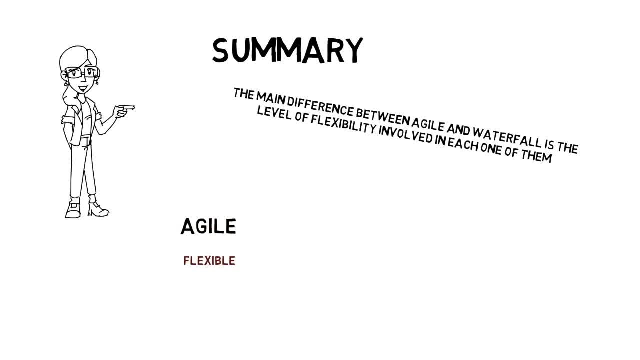 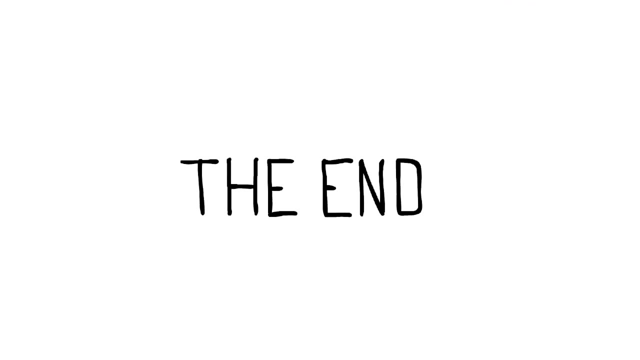 Where agile prides itself as being an approach that is flexible and continuously evolving, waterfall is known to be more rigid and stricter in terms of process structure. Thank you, Thank you.